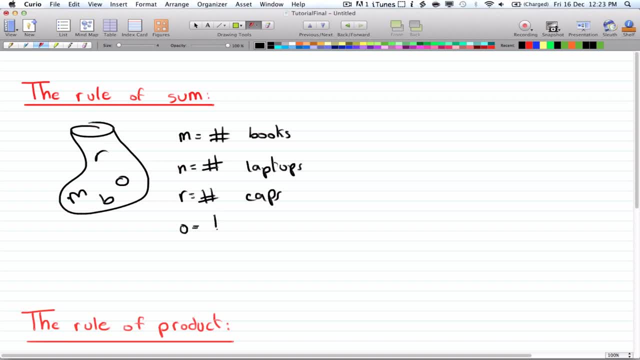 caps and O is the number of speakers, And you want to find how many ways. if you put your hand in and you pick one at random, what's the possibility or how many ways are there to get a different answer. And this is simply M plus N. 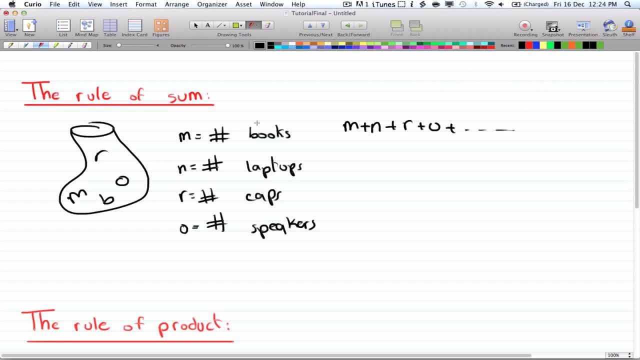 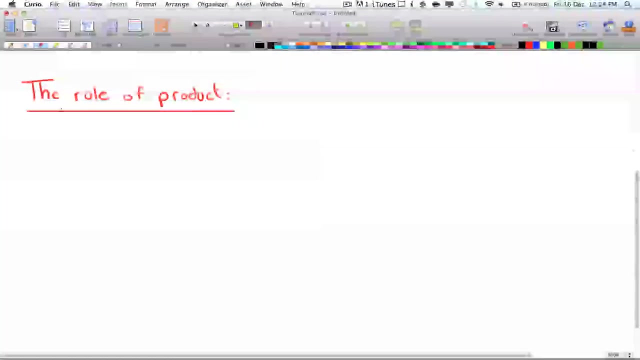 plus R, plus O, plus however many numbers there are, So that's going to be equal to the number of ways to choose one at random. Now the rule of sum is a bit different. In this case, each one is in a bag. So if you have a bag of 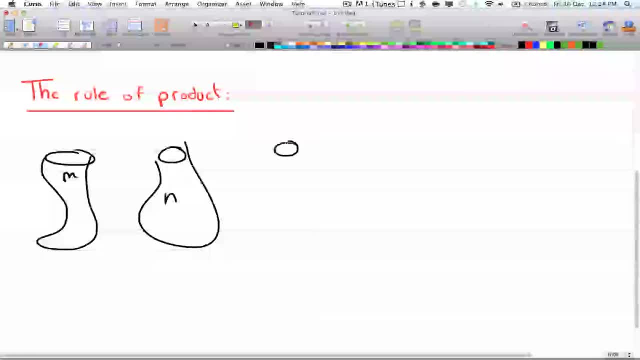 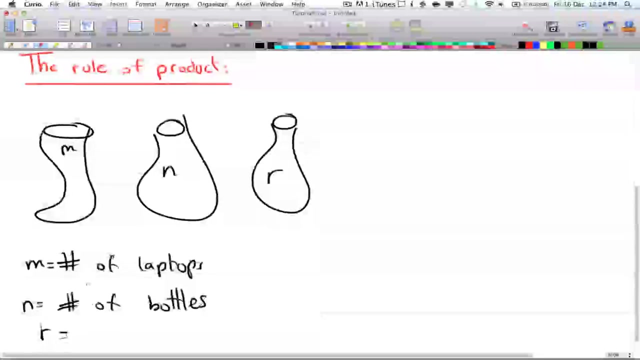 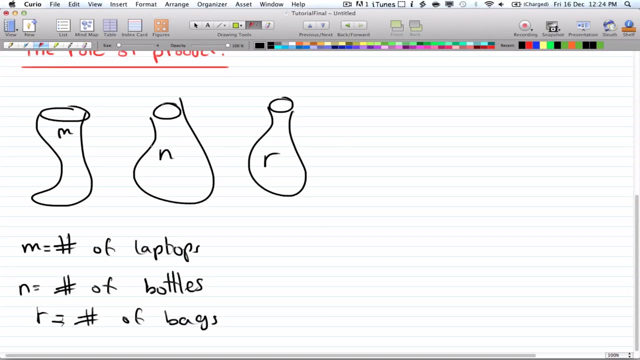 M, a bag of N and a bag of R, and let's say M is equal to the number of laptops and is the number of, let's say, bottles, and R is equal to the number of bags. So in this case you have to pick M first. 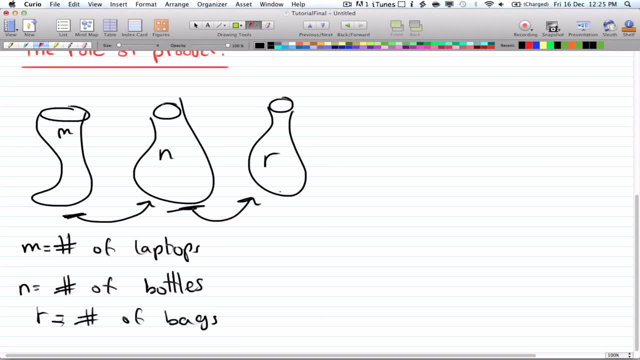 and then you can choose N and then you can choose R. So in this case, you're going to have M times, N times, R times. however many other bags there are, And this is going to give you the number of ways to choose one of each. 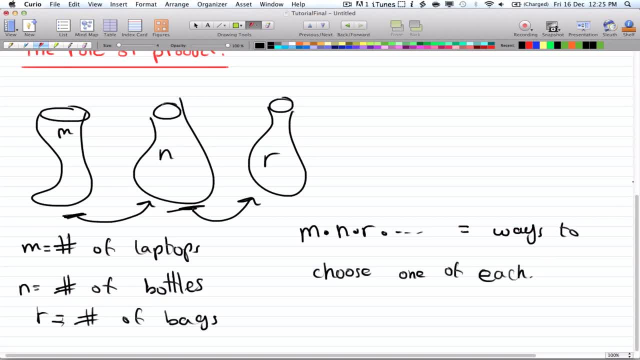 And remember that the rule of product has to be cut into steps. So in this case we choose M first and then N and then R. So this is like step one, step two and step three. However, in the rule of sum it was just all in one step. 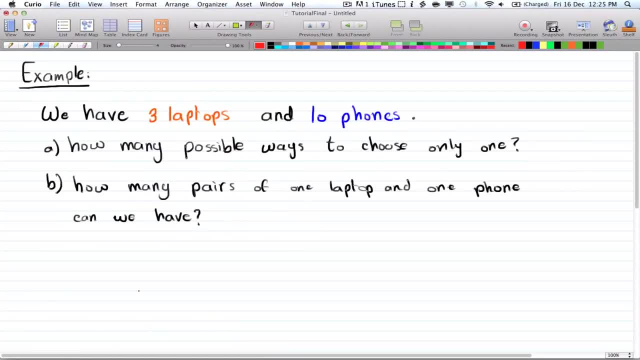 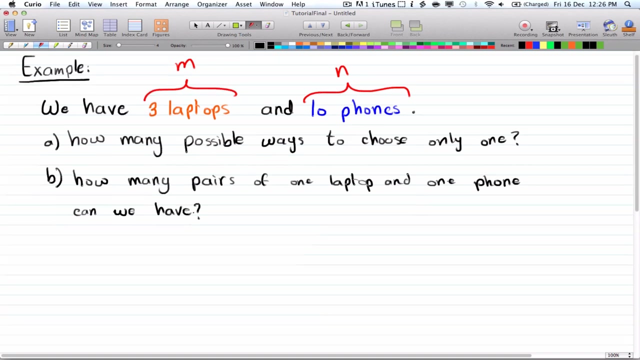 Now let's look at some examples. And here we have the number of bags, And here we have three laptops and ten phones. So let's label them M and N, And we want to find the possible ways to choose only one of them. 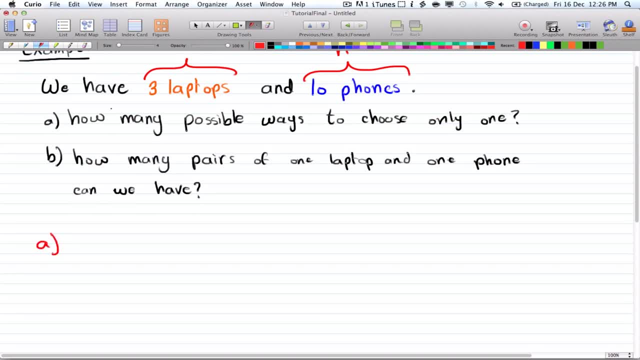 And this is the same as what we did earlier. We have just one bag, So the magical bag that has three laptops and ten phones. So if you just put your hand at random, you're going to have three plus ten. See what's the thirteen ways. 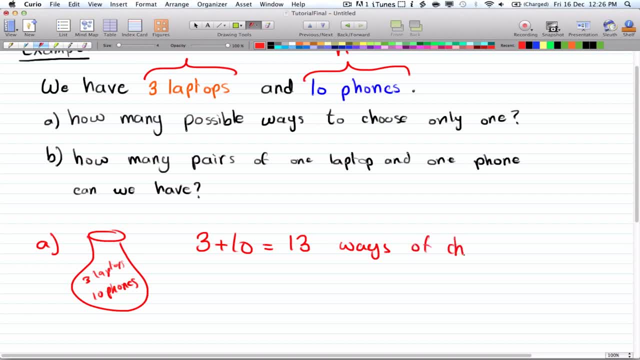 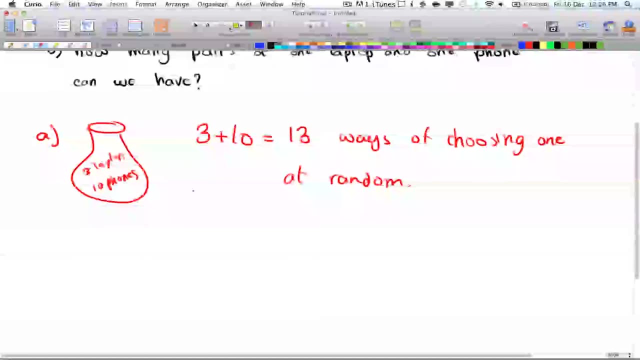 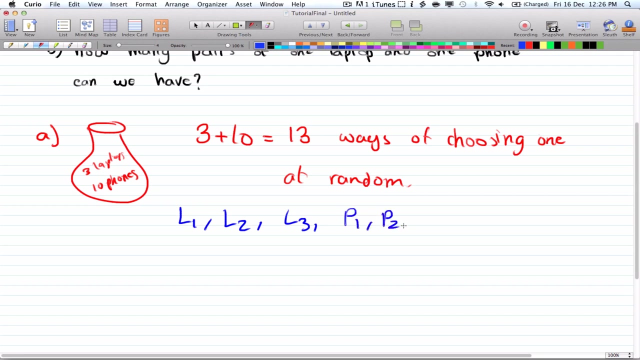 of choosing one of them at random, At random. So if you think about it you can actually say: if you put your hand once, you can get, say, laptop one or laptop two Or laptop three Or phone one Or phone two. 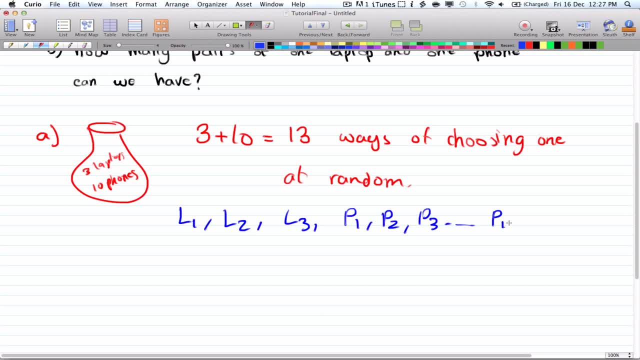 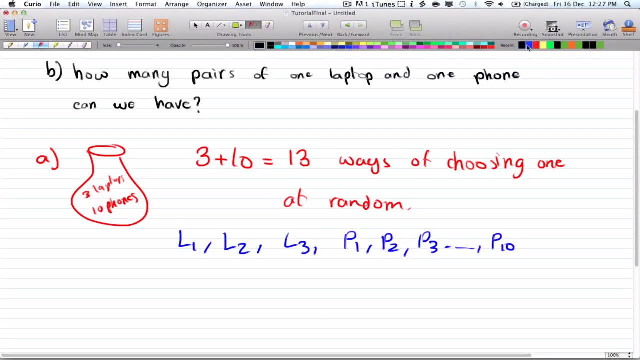 Or phone three, All the way till phone ten, And this will add up to thirteen numbers. And now for B We have: how many pairs of one laptop and one phone can we have? So in this case, we have two bags, One that has um, which one was first. 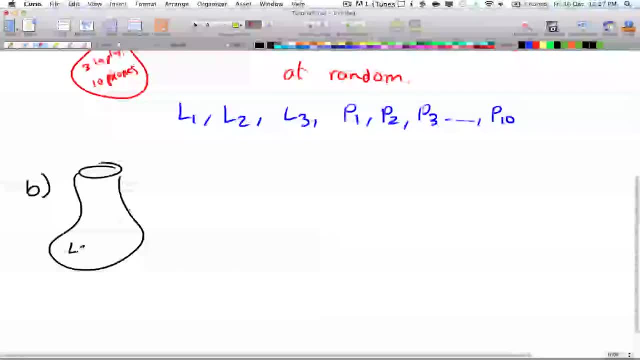 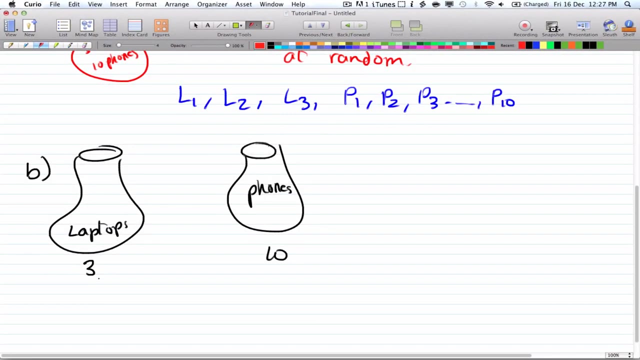 One that has laptops. So this bag has laptops And this bag has phones. So we know that there are three laptops and there are ten phones. So if we choose, um, let's say we picked laptop one, Then on for phones. there are ten other possibilities. 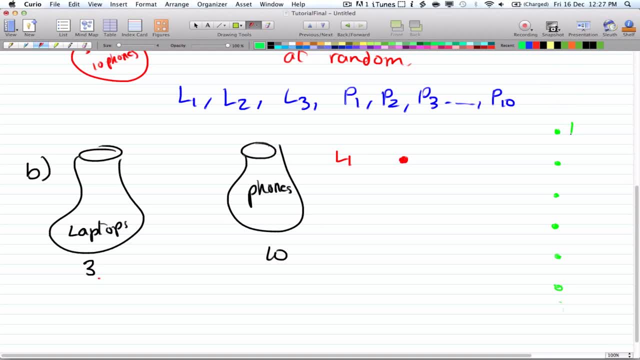 or choices of phones. So we have um phone one, phone two, phone three, phone four, All the way till phone ten. And here we have. we can have laptop one, phone one. So that's one pair, Laptop one, phone one. 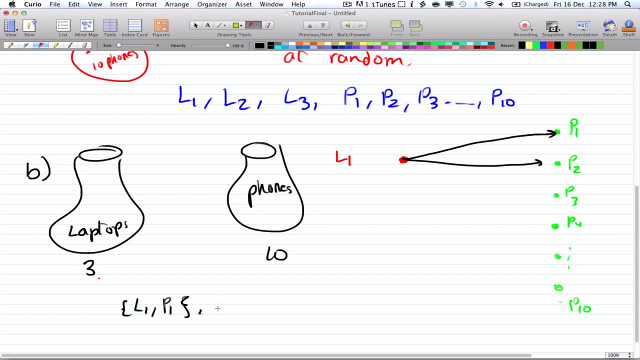 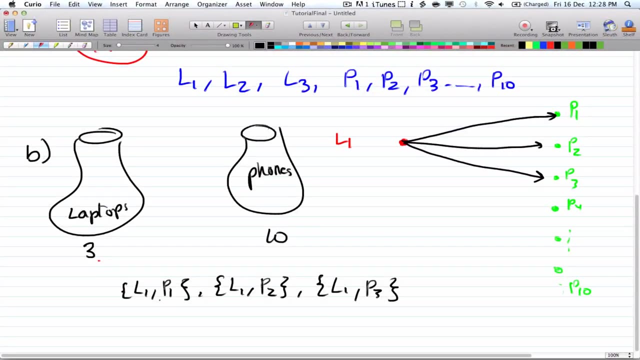 Or laptop one phone two, Laptop one, phone two, Laptop one, phone two. Or laptop three, laptop one, phone three. And if we keep on doing this, um, all we're gonna have is, however, number is in bag one.